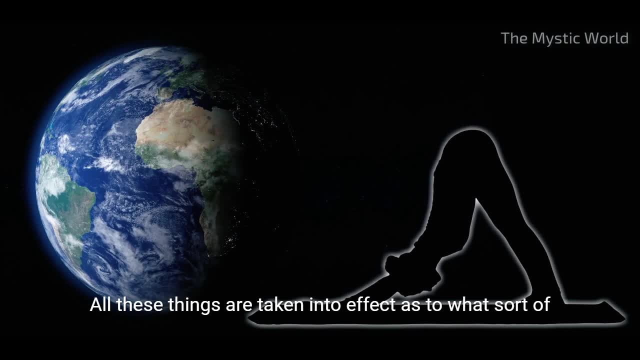 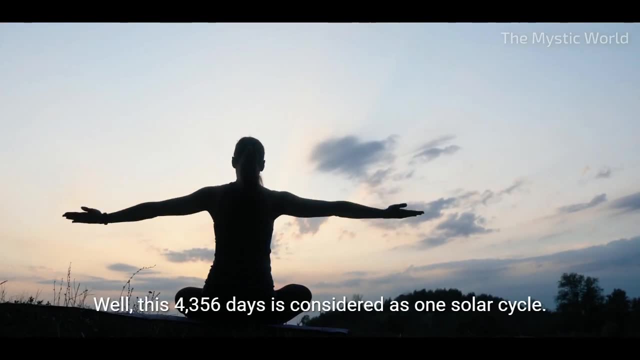 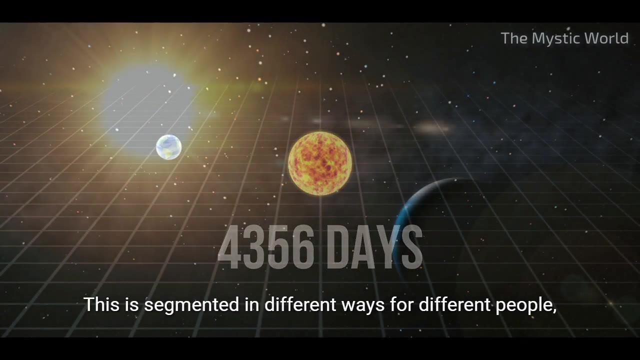 towards its closeness to the sun. all these things are taken into effect. as to what sort of practices you do When I say hatha yoga, this sun and moon, well, this 4356 days is considered as one solar cycle. This is segmented in different ways, for different people, For householders, it's segmented. 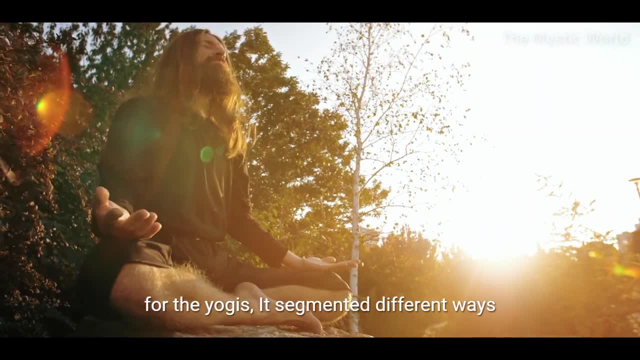 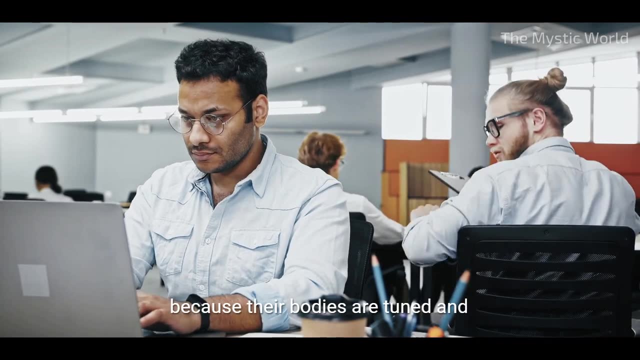 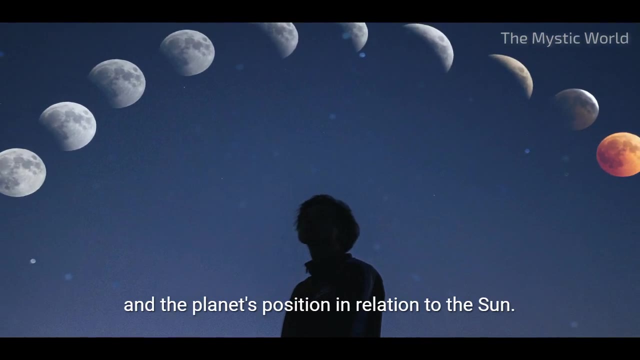 one way. for the yogis it's segmented different ways. for the ascetics one way and people who are into regular worldly life another way, because their bodies are tuned and they need to function differently. Accordingly, the calendar is used depending upon the moon phases and the our, the planet's. 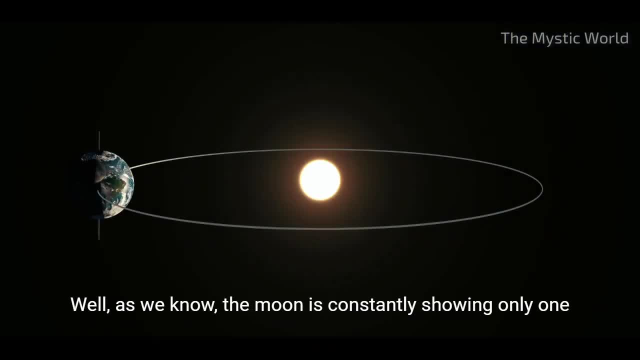 position in relation to the sun. Well, as we know, the moon is constantly showing only one phase to us. It is its rotation is synchronized with planet's rotation, so we're seeing only one phase of the moon. This also is significant because 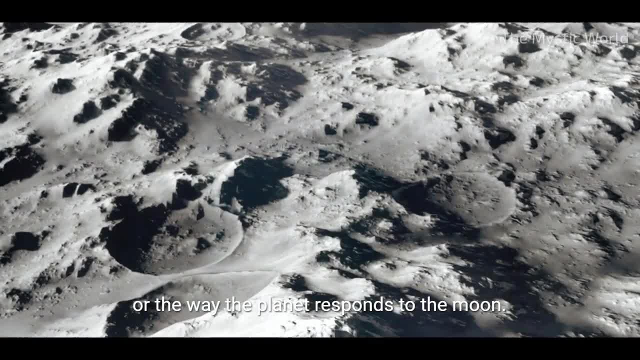 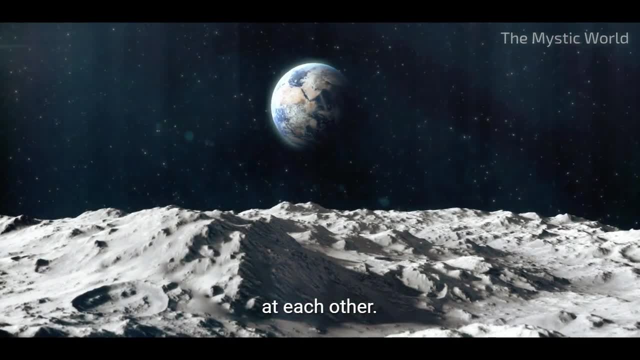 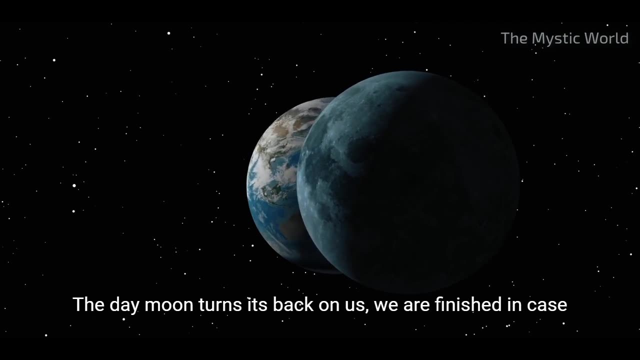 the way the moon responds or the way the planet responds to the moon. there are very wonderful stories how they're always looking at each other. the moon never turns its back upon the planet. the day moon turns its back on us, we're finished, You know, in case the moon turns its back on us. 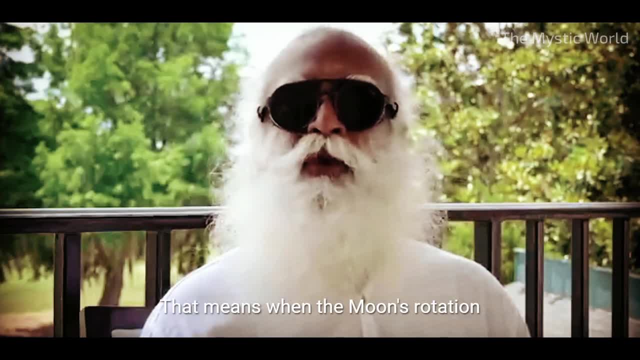 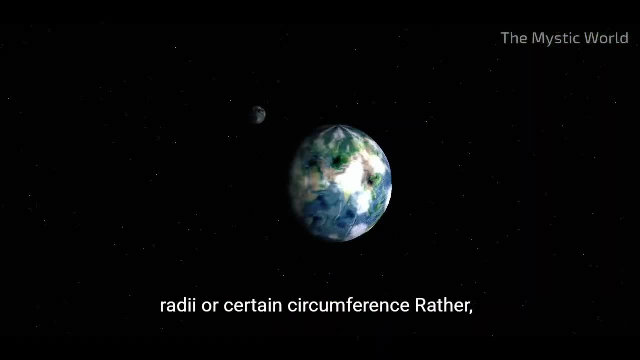 that means human reproductive system will go away and it's over. That means when the moon's rotation goes beyond a certain certain rate of rotation or radii or certain circumference. rather then it will start showing the other face to you. When it shows the other face, that means the end of humanity has come. 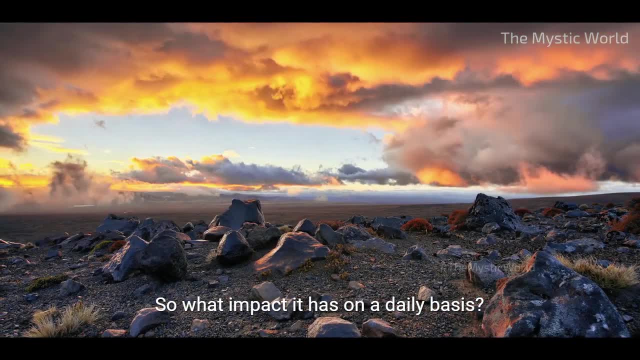 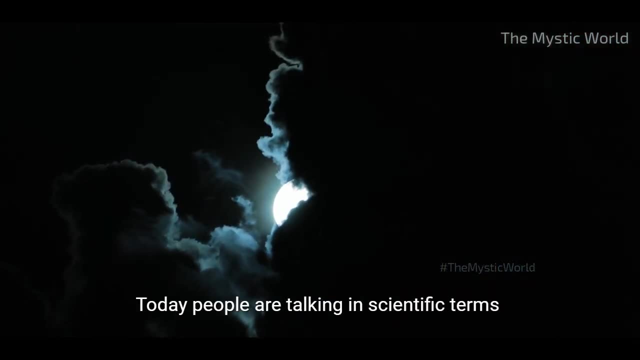 In a few years it will go down. So what impact it has on a daily basis? Well, it is not the moonlight alone, It is a whole…. Today, people are talking in scientific terms of electrical charges, electromagnetic impact and other things. 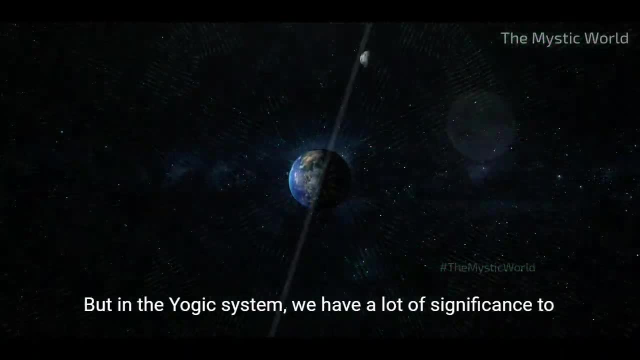 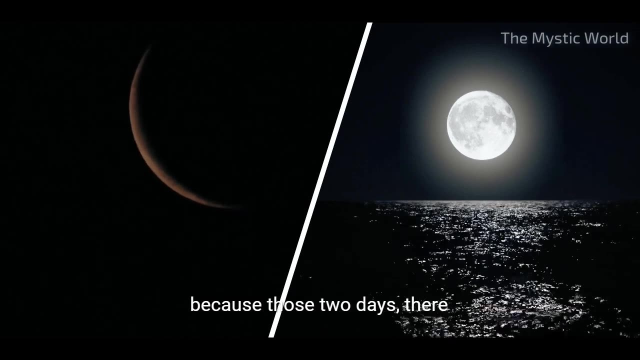 Well, I don't want to talk about it that I am not an expert in that. But in the yogic system we have a lot of significance to full moon and new moon days because those two days there are different types of practices we do. 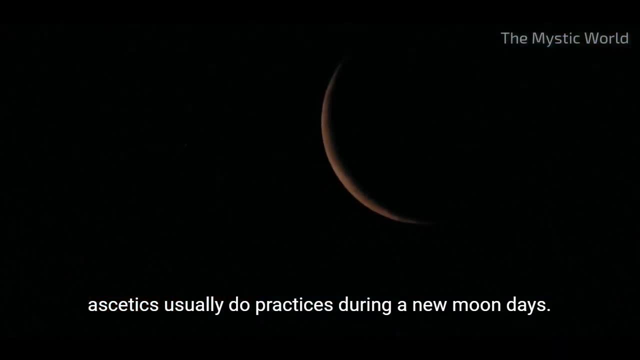 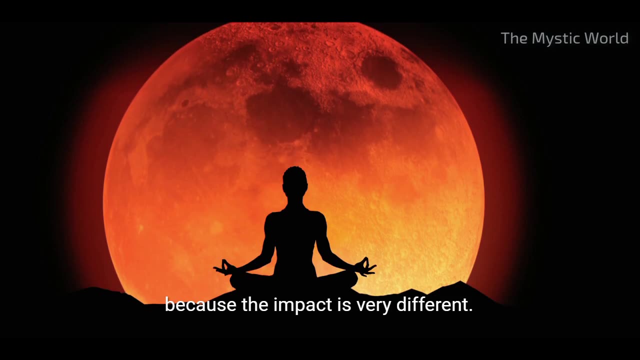 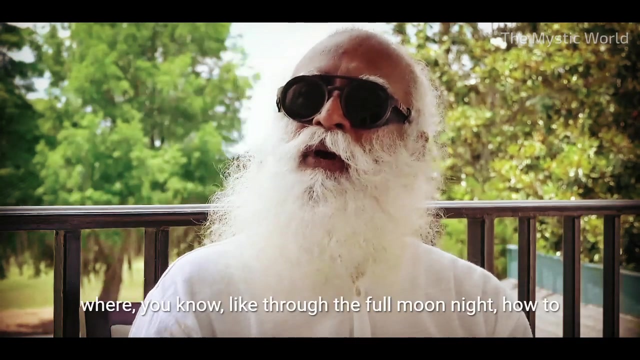 Ascetics usually do practices during new moon days. People in the family way of life. they will do all their practices during the full moon night because the impact is very different. There are variety of devices that we create. I created at one time where you know, like through the full moon night, how to expose. 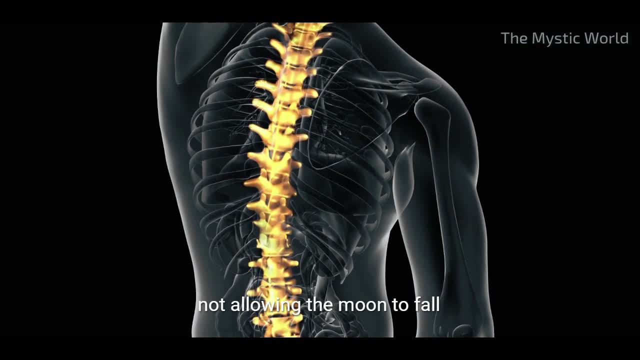 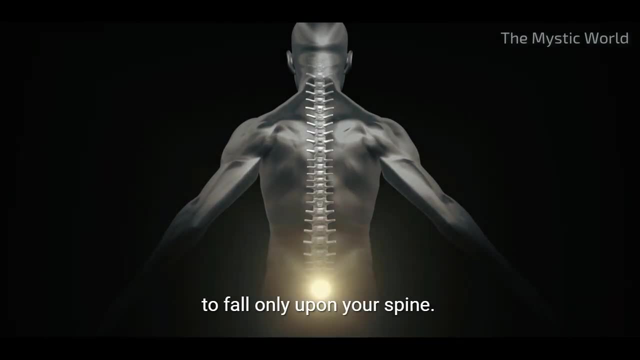 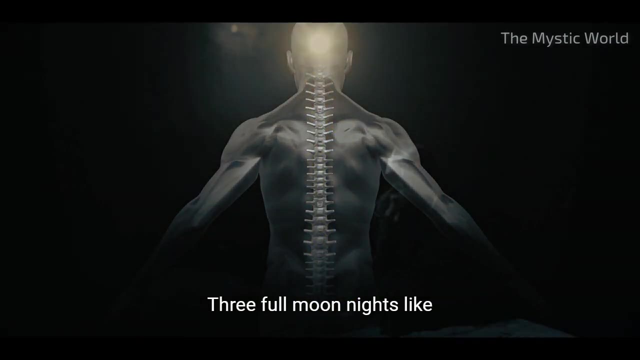 your spine to the moon, not allowing the moon to fall on the other parts of the body, a device so that an arrow crack which allows moonlight to fall only upon your spine, and how it reorganizes your system. Three moon… Full moon nights like that could completely reorganize your system, from ill health to 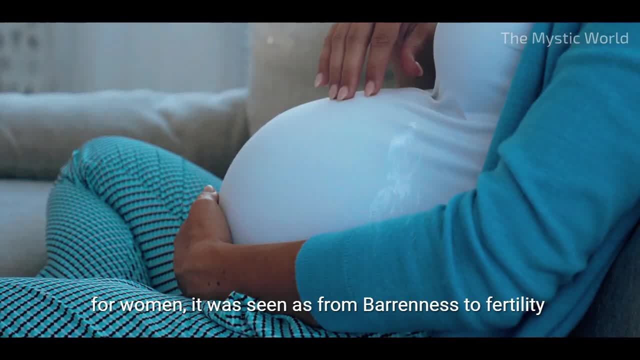 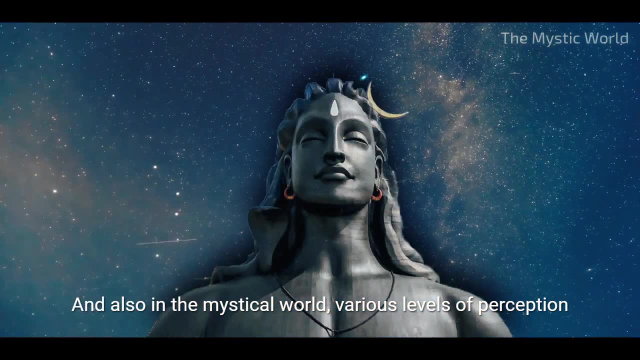 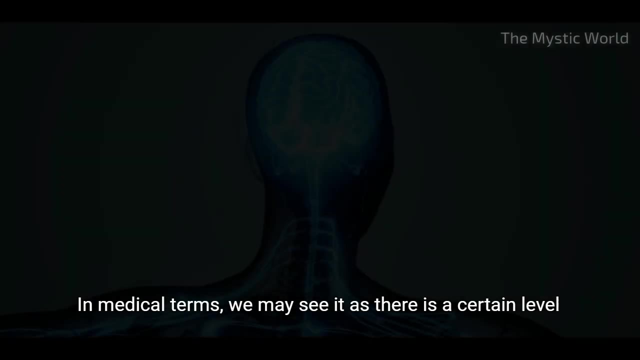 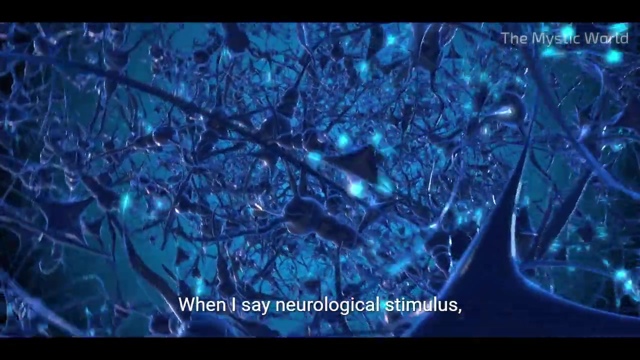 health from… For…. For women it was seen as from barrenness to fertility and various other aspects, and also in the mystical world, various levels of perception were always, you know, connected with the moon. In medical terms, we may see it as there is a certain level of neurological stimulus. 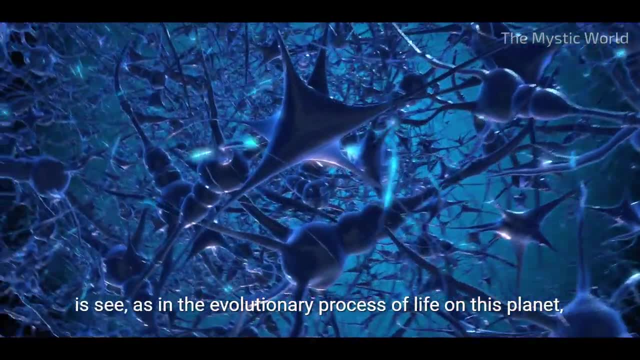 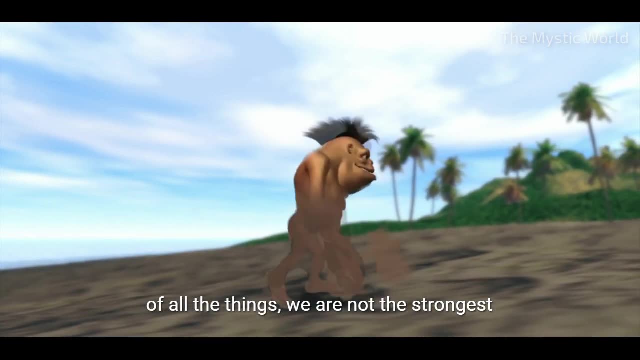 When I say neurological stimulus, why I am talking about this is see, as in the evolutionary process of life on this planet. Of all the things, we are not the strongest creature on this planet, but we have the most complex and sophisticated neurological system. 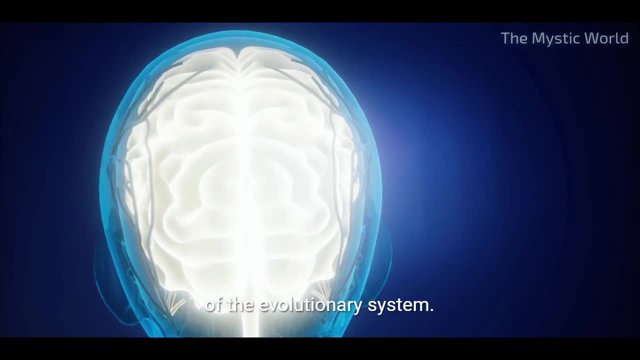 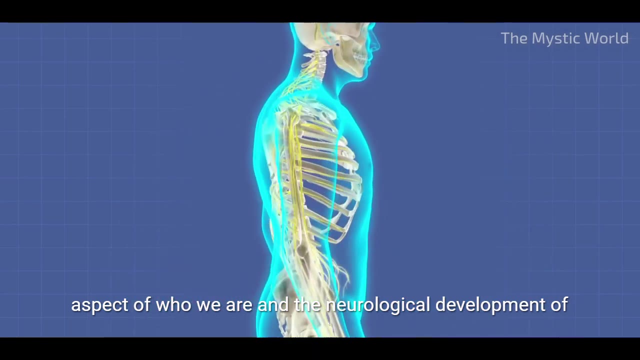 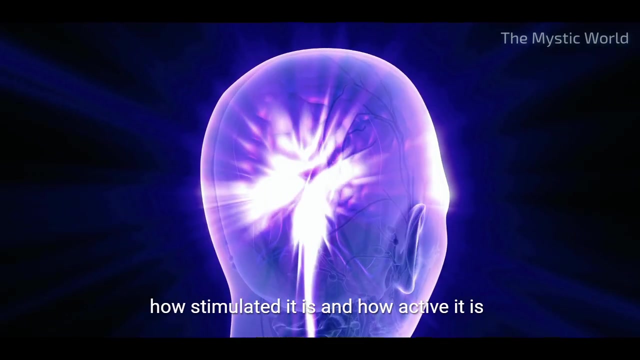 That's what renders us as really on top of the pile of the evolutionary system. So this neurological development is the most significant aspect of who we are, and the neurological development of the human being and how stimulated it is and how activi… activities and how. 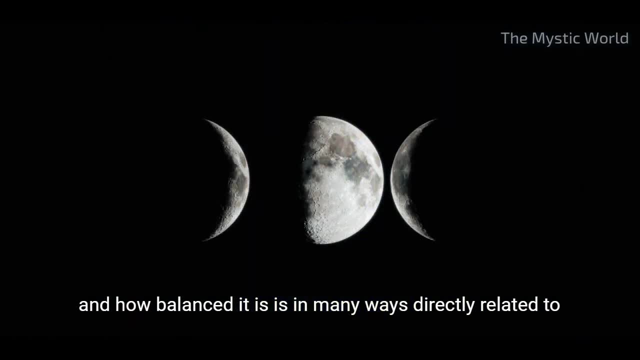 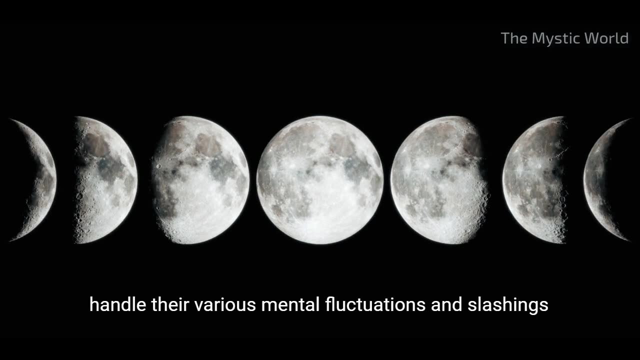 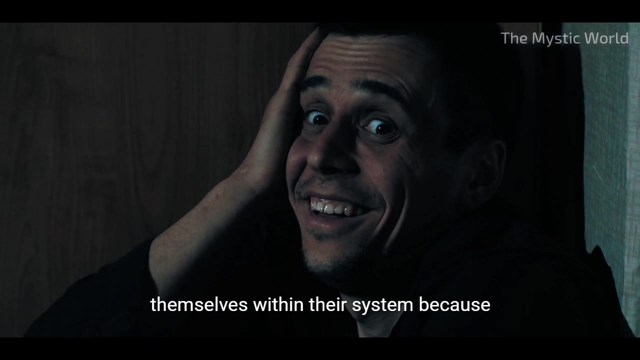 balanced it is is… Yeah, And in many ways directly related to the faces of the moon, and there are very many ways in which people can make use of it to handle their various mental fluctuations and sloshings that they have. You know, many human beings go into tides themselves within their system because the 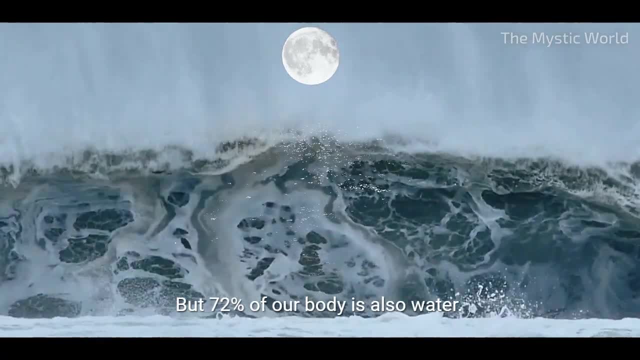 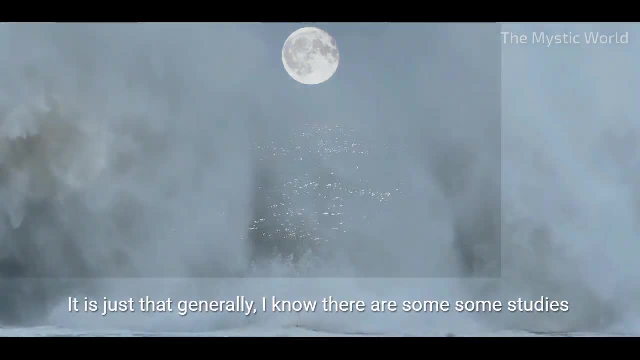 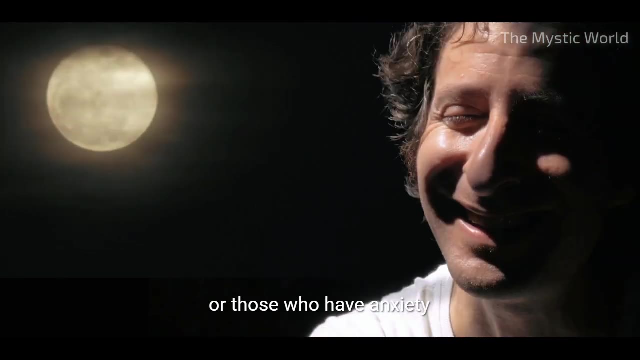 whole oceans are going up, but seventy… seventy-two percent of our body is also water, So there is fluctuation in the system. it is just that generally. I know there are some studies saying on this day people tend to become more imbalanced, or those who have anxiety. 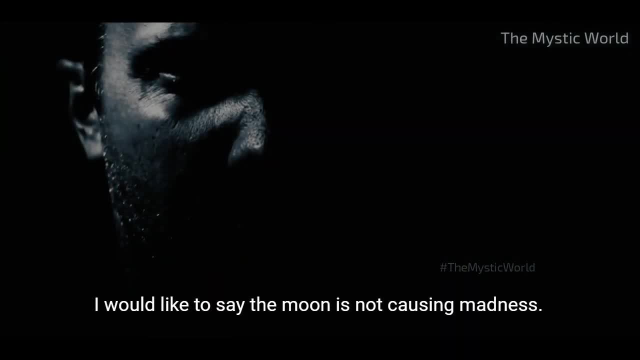 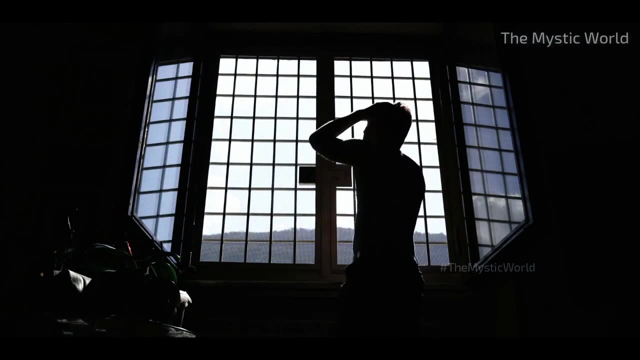 and manic depressions go off control. this kind of things. I would like to say: the moon is not causing madness. I am saying this so that moon is liberated from this word. Lunar means if you say loony, people think you are mad. all right. 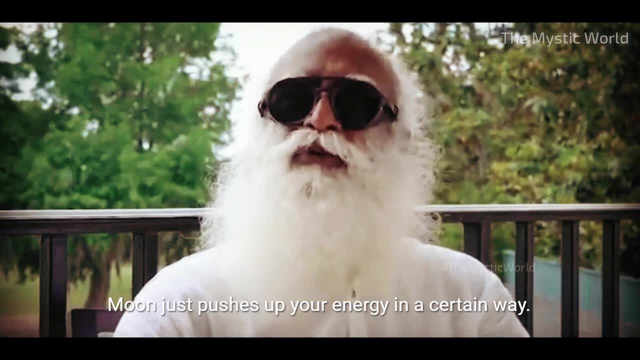 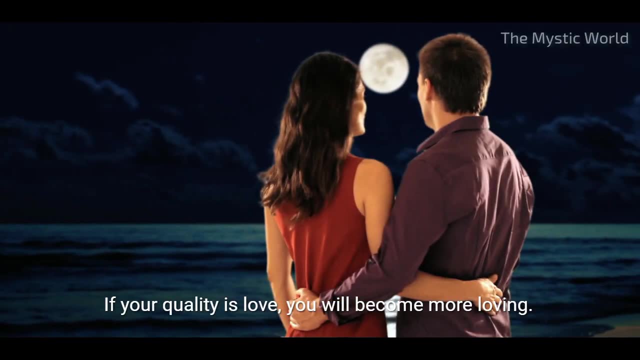 So moon does not cause madness, Moon just pushes up your energy in a certain way. If your quality is joy… you will become more joyful. If your quality is love, you will become more loving. If you are meditative, you will become more meditative. 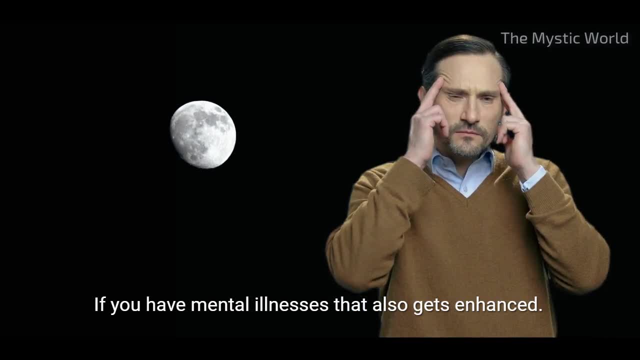 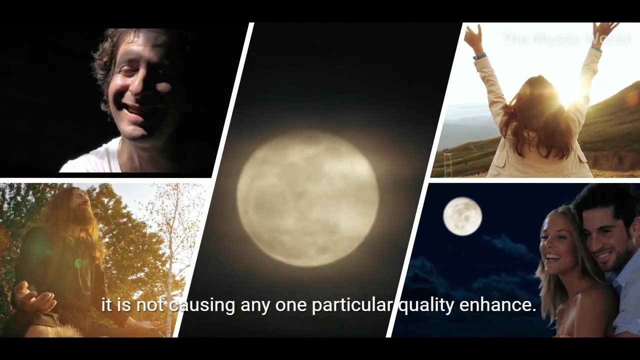 If you have mental illnesses, that also gets enhanced. Whatever is, your quality gets enhanced because of full moon. It is not causing any one particular quality in us. it definitely does not bring about madness. It is just that it enhances who you are on that day. 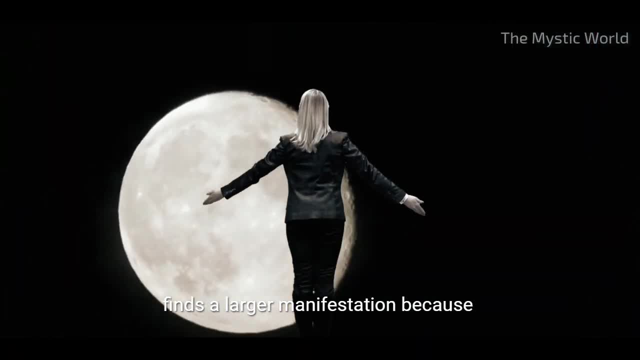 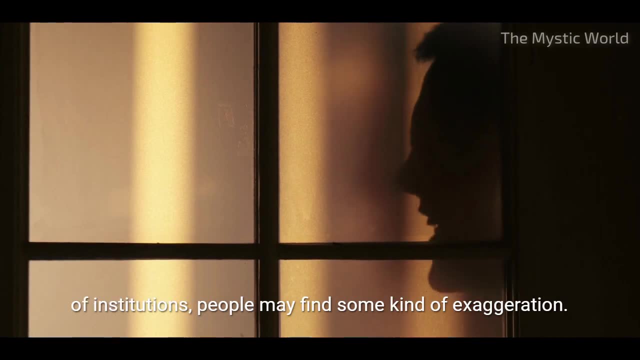 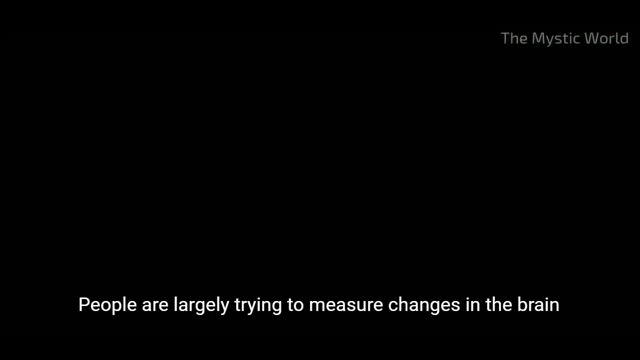 Whatever is your quality finds a larger manifestation Because of that. maybe in the medical institutions, mental and other kinds of institutions people may find some kind of exaggeration on those days. People are largely trying to measure changes in the brain activity and stuff like that. 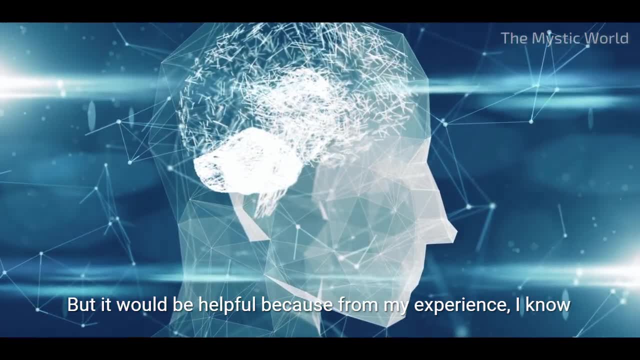 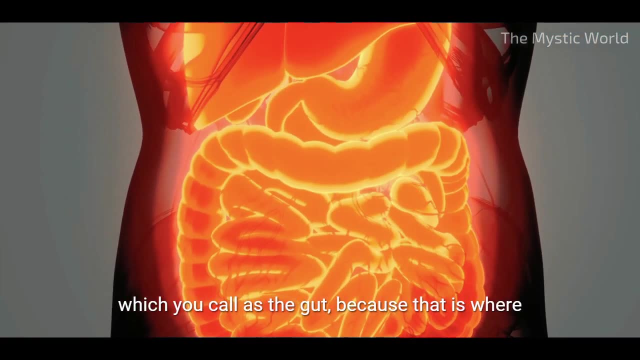 But it would be helpful because from my experience I know that the maximum amount of change happens in your belly, in this region which you call as the gut, because that is where the real change happens and it has consequences in the brain and the rest of the body. 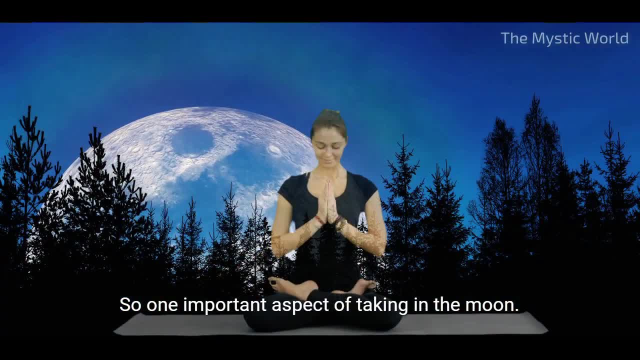 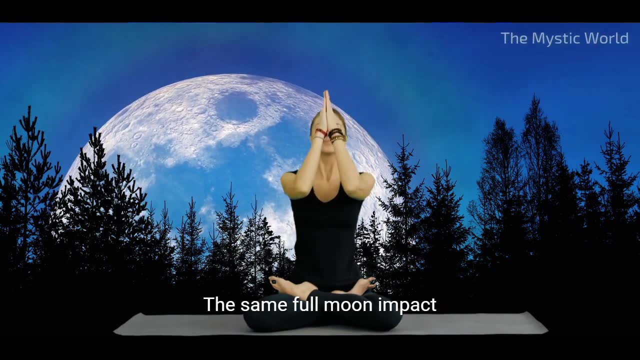 So one important aspect of taking in the moon. there are practices in yoga where you can live like every day In your experience. it's like full moon. The same full moon impact is on in your body on a daily basis. there's a whole lot of practices. 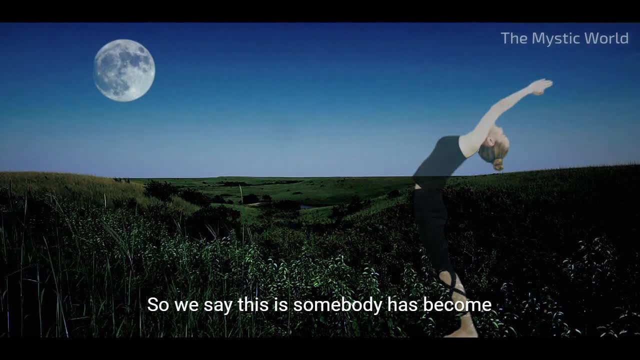 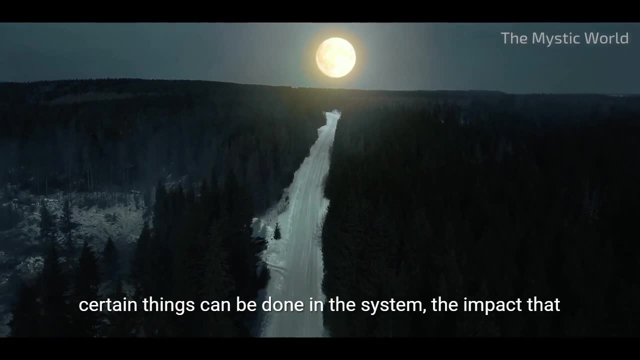 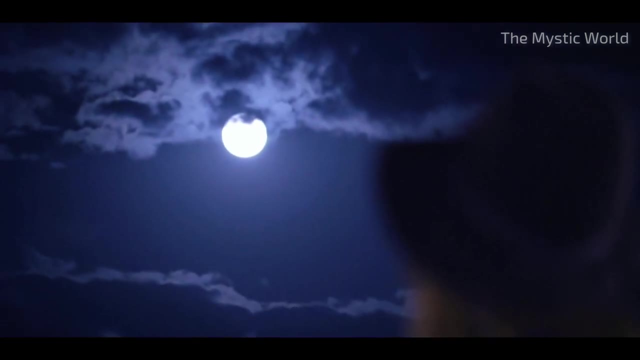 like that. So we say this is a…. somebody has become like an eternal moon within himself, that is like a full moon always. Suppose certain things can be done in the system, the impact that the full moon has on various aspects of your body, the cellular behavior in the system- this can be replicated.